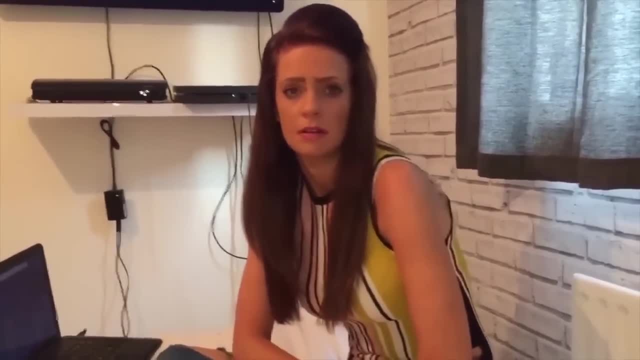 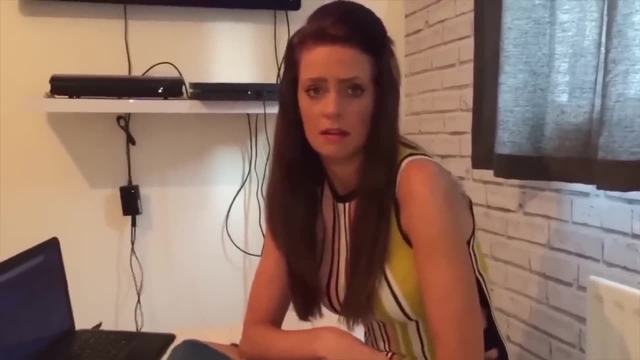 you could eat 12?? No, So you don't think you could eat 12.. So what pizza would you have? by the way, Hawaiian, So you'd have a Hawaiian large pizza cut into 8 slices rather than 12? Yeah, Because you could only eat 8 slices. Yeah, because I can't eat the extra 4.. 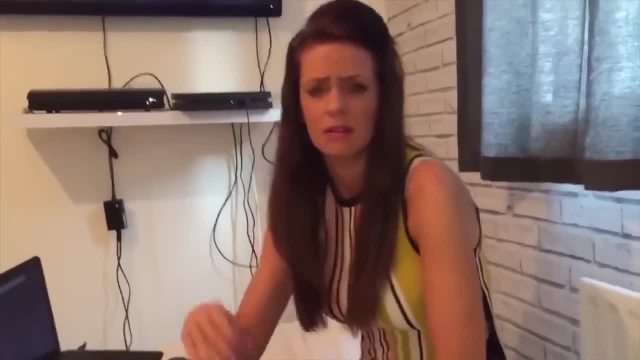 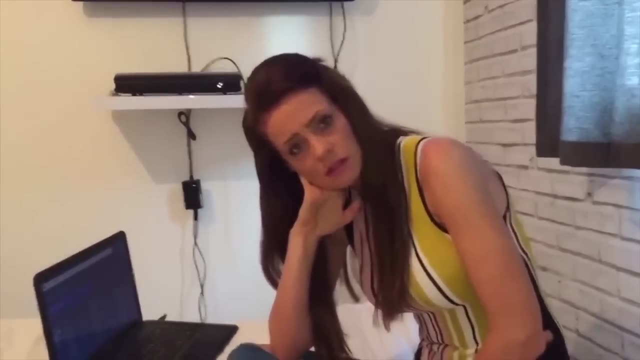 Why are you laughing for? Let me get this straight. yeah, You're telling me that you would order a large Hawaiian pizza and you'd have it cut into 8 slices because you couldn't eat 12 at the same pizza. Yeah, because I can't eat the extra 4 slices. Brad, I'm not. 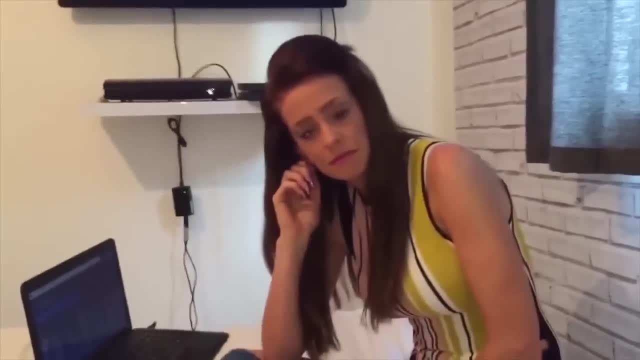 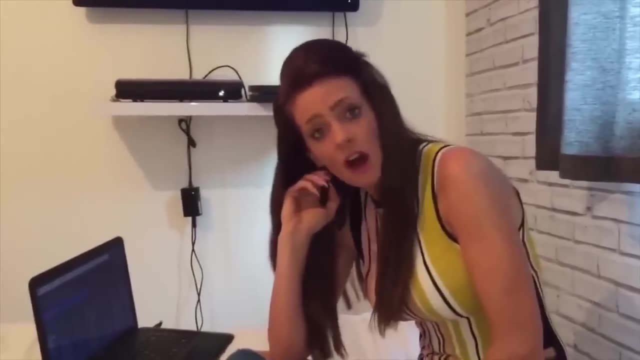 fat and gutty. Why are you laughing? You'd have 8 pizza slices. yeah, Of a pizza, I'd have 8,. Brad, because what? This is what bugs me about you. You're not understanding what I'm saying. You're not understanding what I'm saying. You're not understanding. 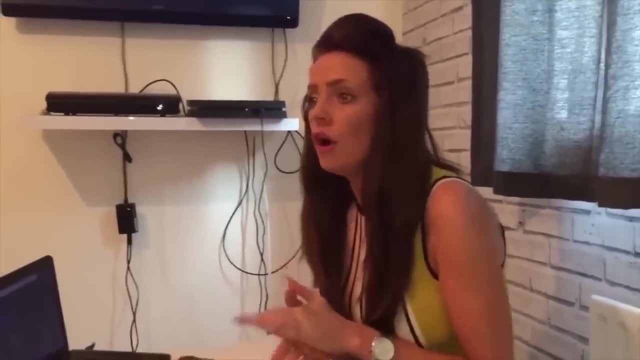 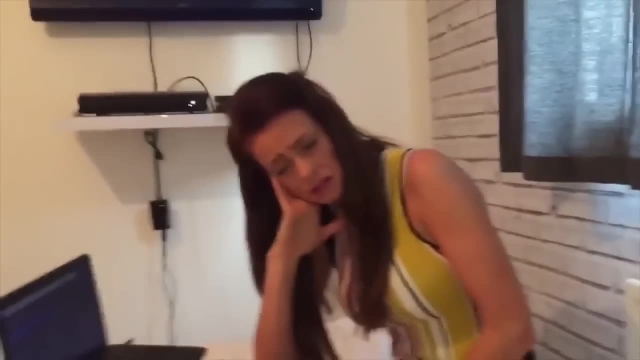 what I'm saying. I'd have 8, yeah, Because I can't eat the extra 4, because that'd be too much for me. Why are you laughing for Din? I'm the Din, Right, so let me get this. 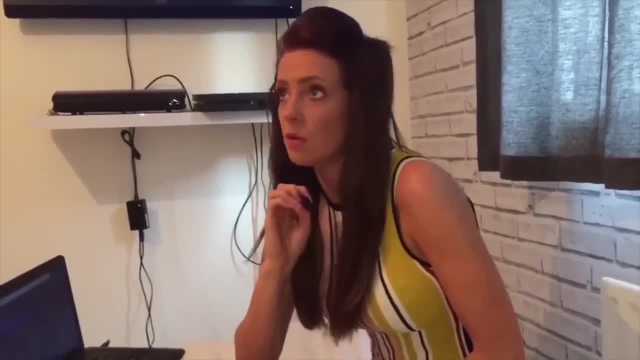 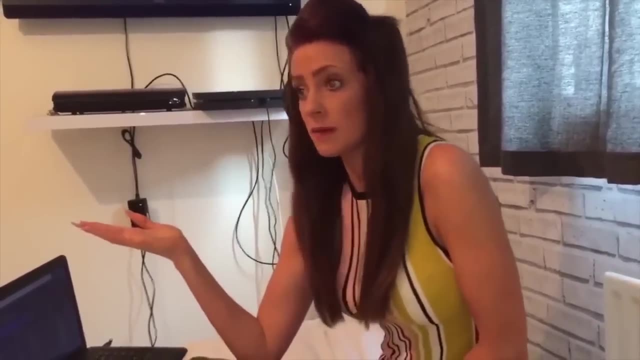 straight: You've got a large pizza. yeah, Yeah, I've got a large Hawaiian pizza. He asked me: Jenny, how many slices would you like that cut into? I say 8, please, sir. And then he comes back and went 8 pieces. And you ask me: why have I done that? Because 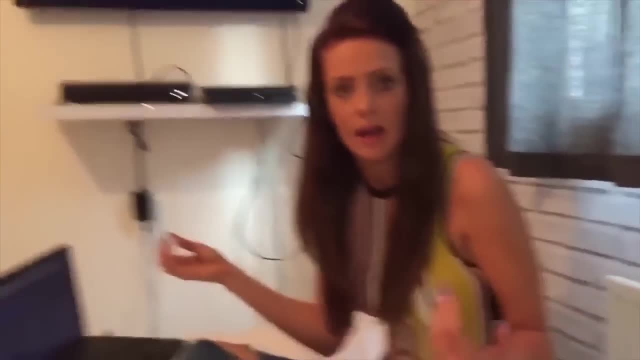 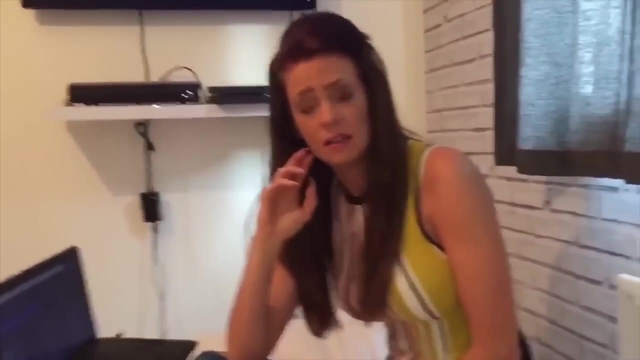 I can't eat the extra 4 bits. What is so hard to understand about that? But it's the same pizza, Jen, so it'd be the same amount, wouldn't it? How would it? There's 4 extra bits of pizza on my plate. You're annoying me now, Right? so would these. 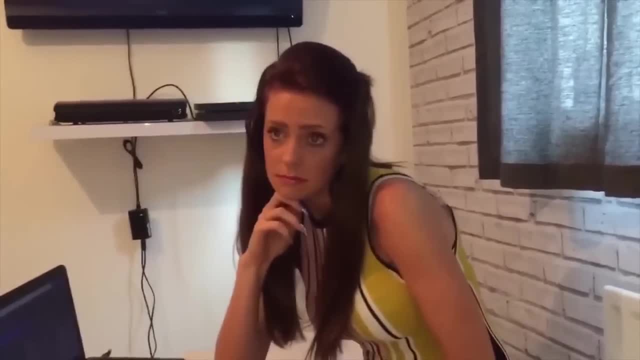 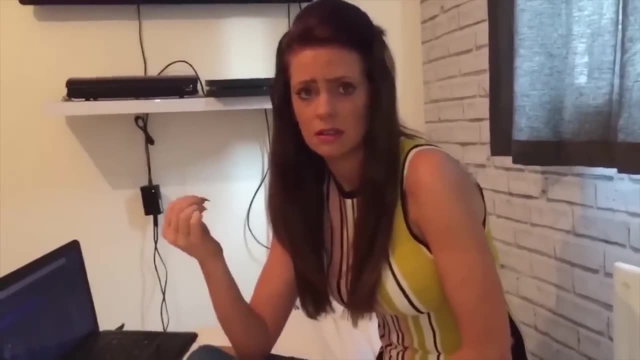 8 slices be the same size as the 12 slices. Oh, I don't know. I don't cut pizza for a living, Brad. No, this is common sense, isn't it? Would they be the same size, Do I cut? 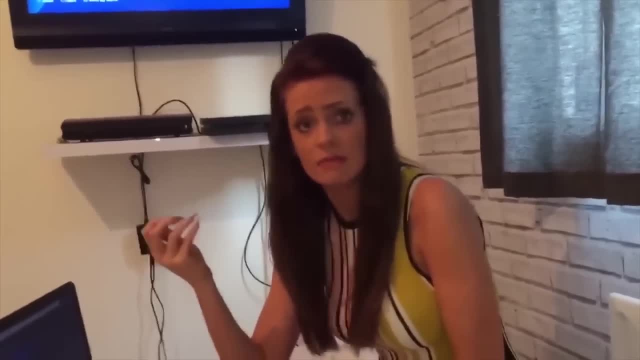 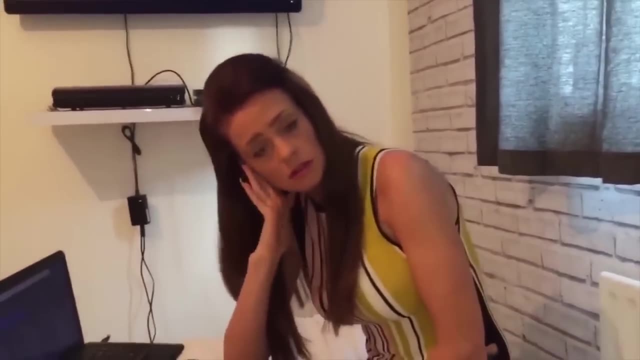 pizza for a living? No, So how am I going to know if they're the same size or not? Do you measure your f***ing pizza when you go to a pizza restaurant? But Jen, it's the same pizza. What are you not getting about this? It's the same pizza, so you'd have. 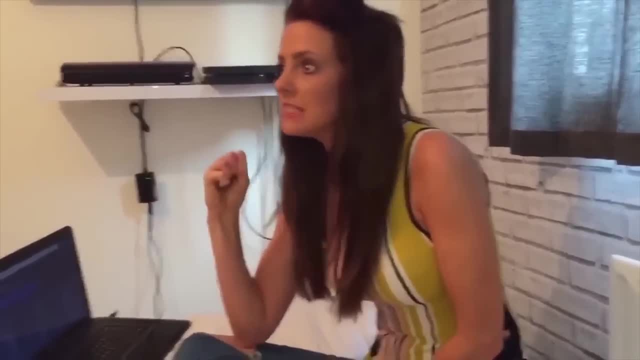 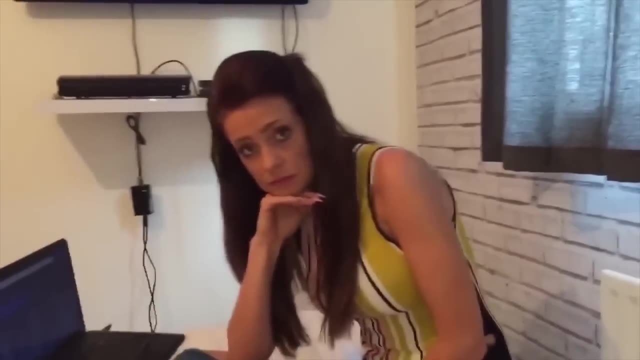 8 over 12,. yeah, Yeah, because I can't eat f***ing 12 bits, Brad, because I can eat 8, but an extra 4 would make me f***ing too full up. You're not getting what I'm saying.